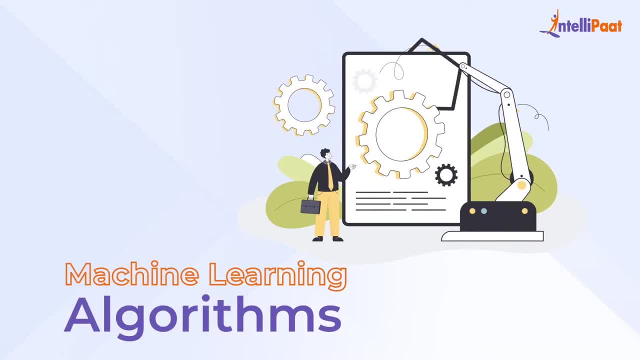 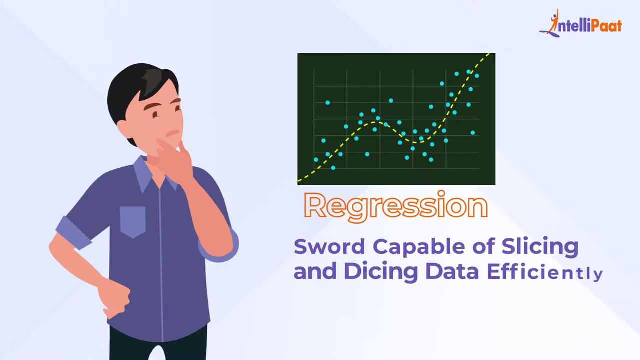 of machine learning algorithms as an armory packed with axes, swords, blades, bows, daggers, etc. You have various tools, but you ought to learn to use them at the right time. As an analogy, think of regression as a sword capable of slicing and dicing data efficiently. 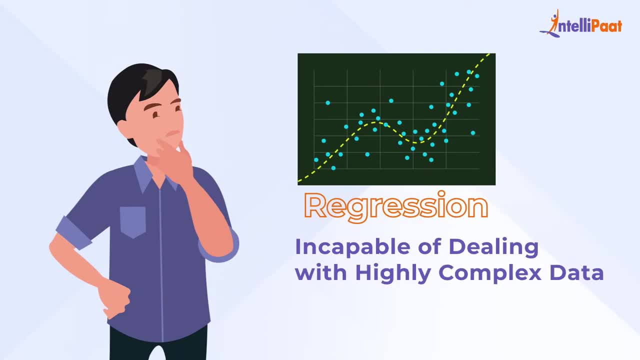 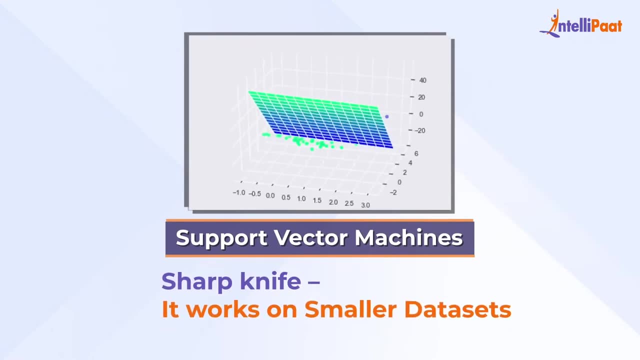 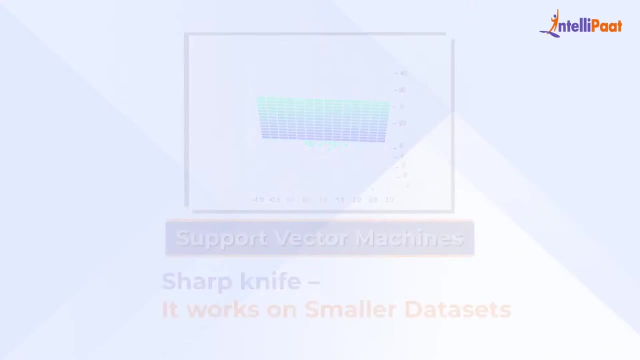 but incapable of dealing with highly complex data. On the contrary, support vector machines is like a sharp knife: It works on smaller datasets, but on complex ones as well. So, that being said, I welcome all of you guys to this session on Support Vector Machine. 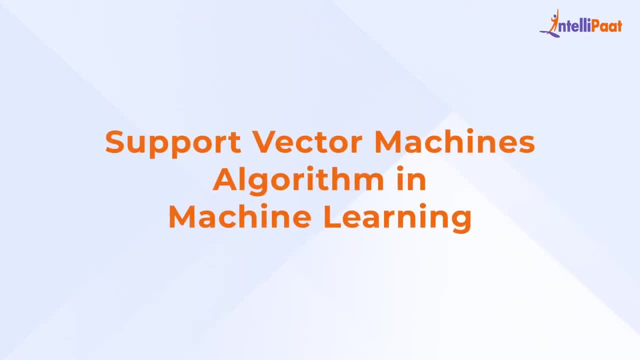 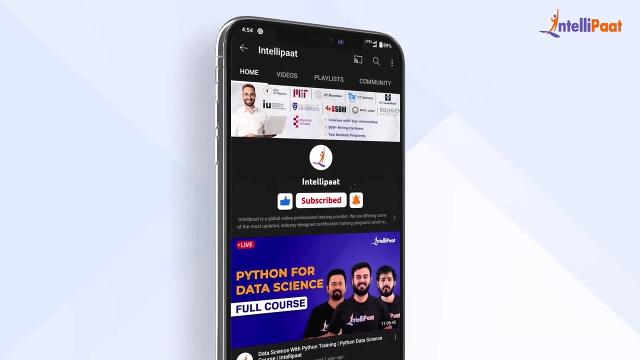 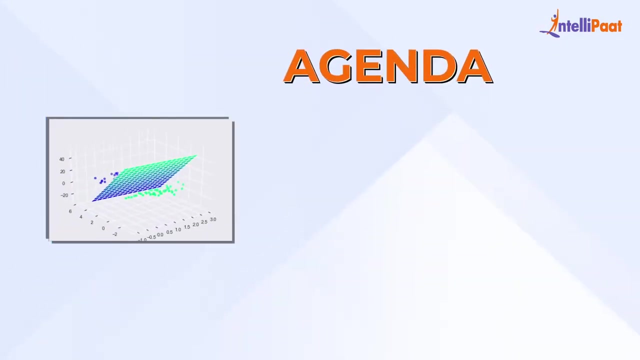 Algorithm in Machine Learning. But before we begin with this session, please make sure that you guys hit the subscribe button and bell icon so that you never miss an update from Intellipaat YouTube channel. First of all, let's discuss the agenda for this session. 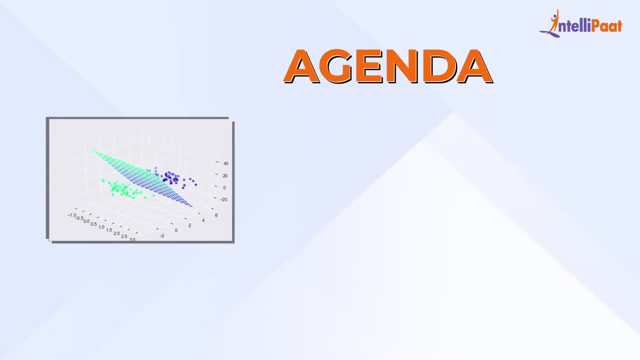 We'll begin this session on a very friendly note by talking about the basic intuition behind the concept of support vector machine. After that, we'll delve into the hands-on demo where we will implement support vector machine algorithm with the help of scikit-learn. 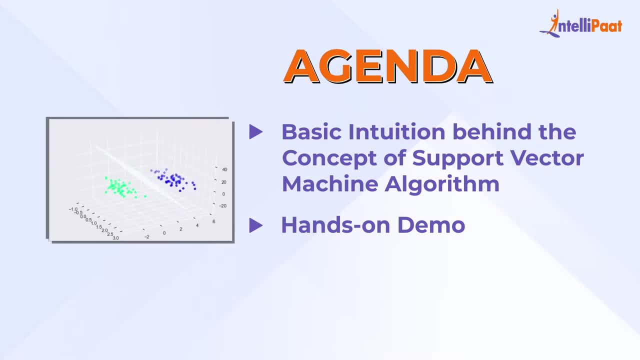 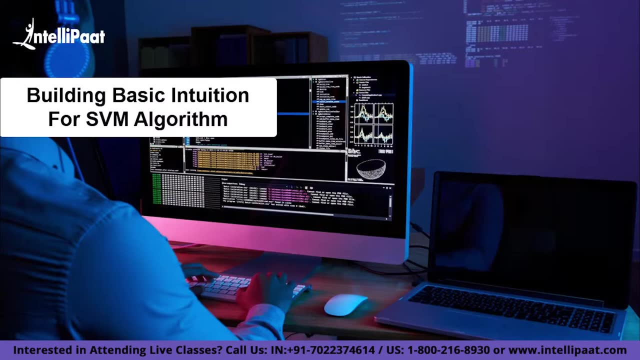 library. I hope all of you guys are clear with the agenda. So, guys, without wasting any time, let's get started with the first topic of this session, that is, building basic intuition for support vector machine. So, guys, without wasting any time, let's get started. 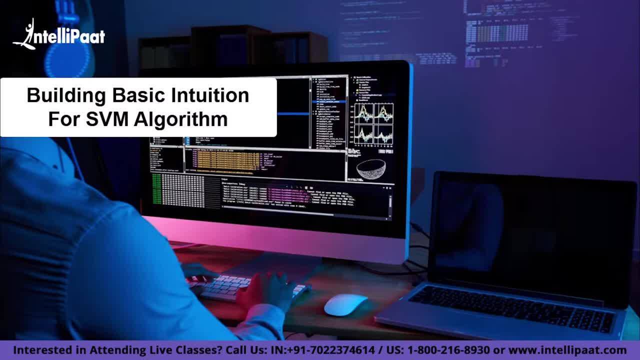 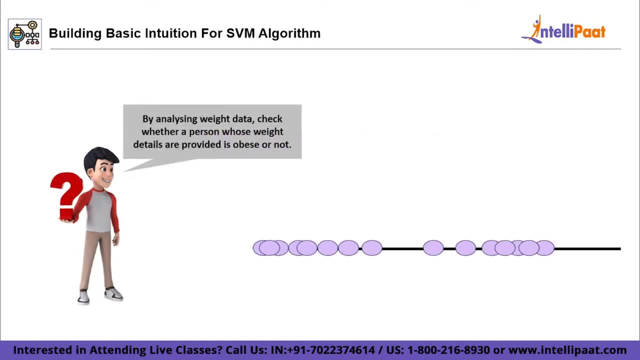 with the first topic of this session, that is, building basic intuition for support vector machine algorithm. To start things off, let's imagine a sample data set where we are given with the weight of few important personnel and we need to predict if a particular person 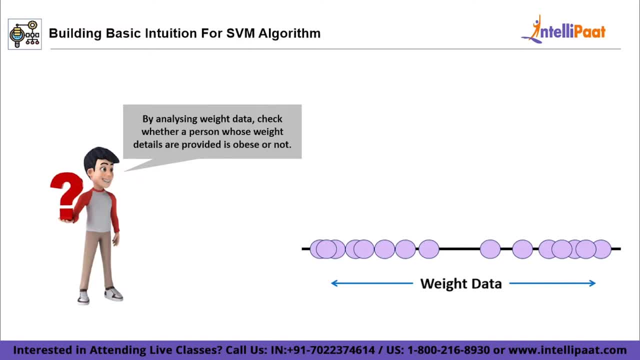 is obese or not. Well, let's say, these red dots represent the people that are not obese and these green dots here represent that these particular dots belong to the category of obese people. Based on this data given here, this data given here, we can decide if given new weight or entry belongs to obese tag or. 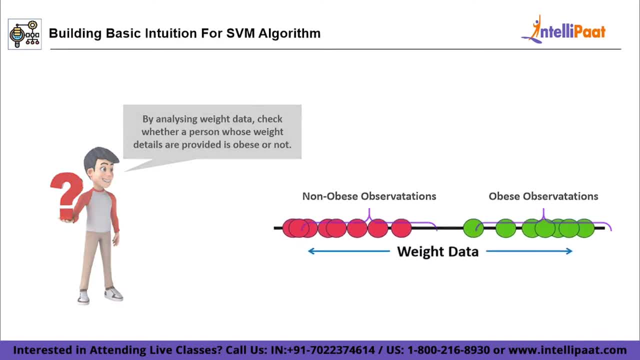 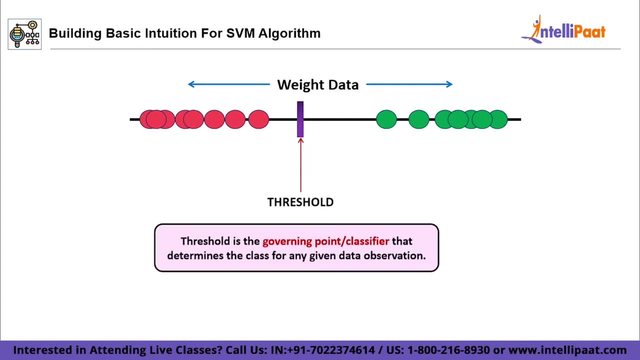 non-obese tag. alright Now. in general, the linear classification approach tries to find a threshold. If the given new observation has a less mass, then it will be considered as a non-obese observation, And other way around if it is greater than that of threshold. 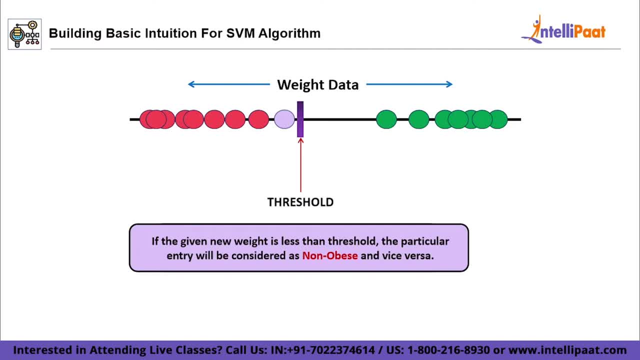 the observation will be said to be as obese observation. But now consider this particular observation. Since this observation has more weight than that of threshold, it will be considered as obese observation. But, guys, this data point is quite closer to the non-obese. 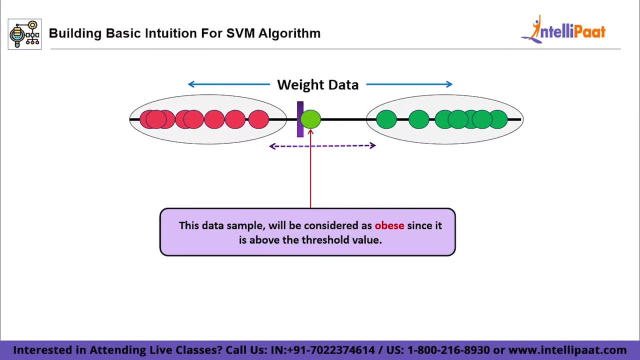 class and very far from the obese class right. So ideally, this data point should be belong to the non-obese label right, and this is where the issue of misclassification arises. This is precisely what we can say as the limitation of basic linear classifier. 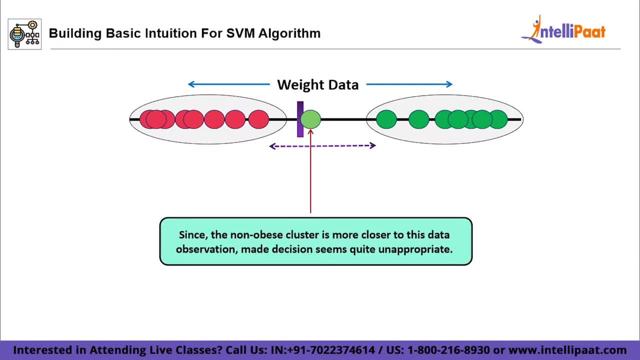 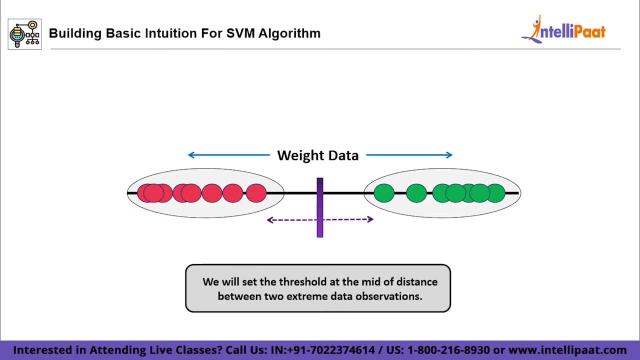 or regressor. Now, can we do better than this? Well, of course yes. The first basic approach we can imply in this particular case is to take an average of distance between the observations on the edge of each cluster and then place a threshold. 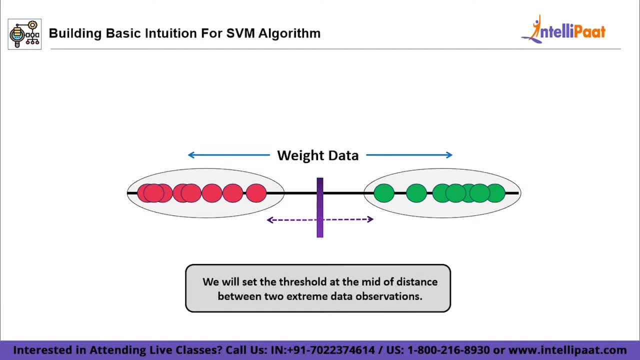 at the mid of them. Now, if I consider this point, a classifier will recognize it as a non-obese observation right, And this is actually solving the problem that we face in last case, study right. One more thing I want you guys to note is the distance between 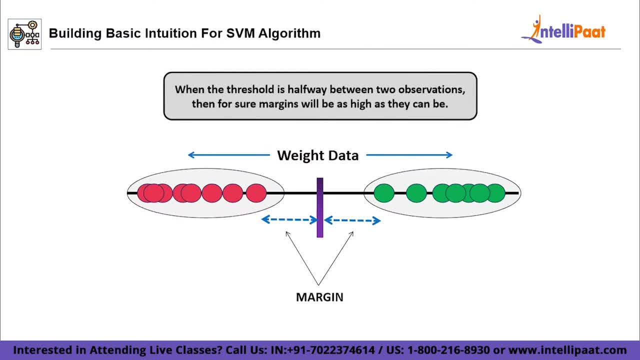 the data point and the threshold is considered as margin and those points will be at the edge of that cluster alright. So basically, by placing the threshold at the middle of edge points of two clusters, we are making sure that the distance between the observations. 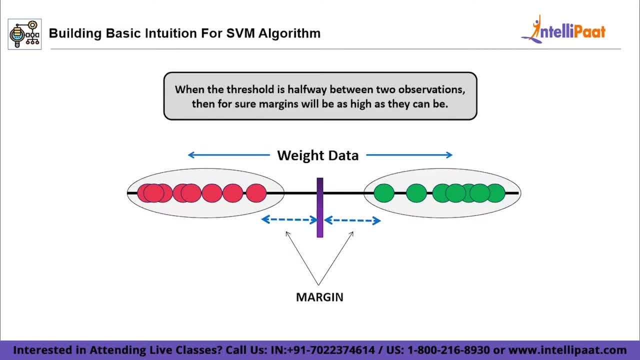 and the threshold are the same and both reflect the margin. Now, when the threshold is halfway between two observation, then for sure margins will be as high as they can be. Alright, And this approach of placing threshold at mid is known as maximum margin discussion. 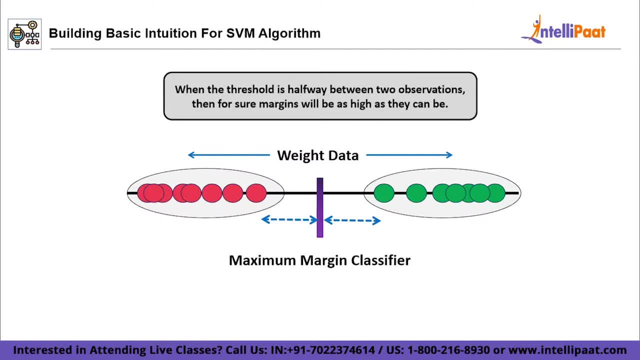 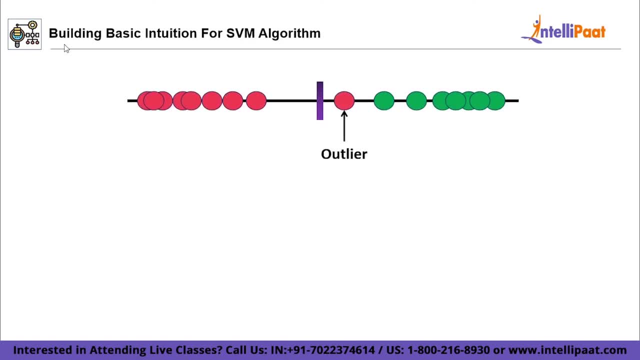 classifier. Well, is this? it? This is the solution that we are looking for? Well, no, let's visualize a slightly different training sample. Let's say: this is our training sample, which contains an outlier that was classified as not obese, but it was much closer to the obese observations. 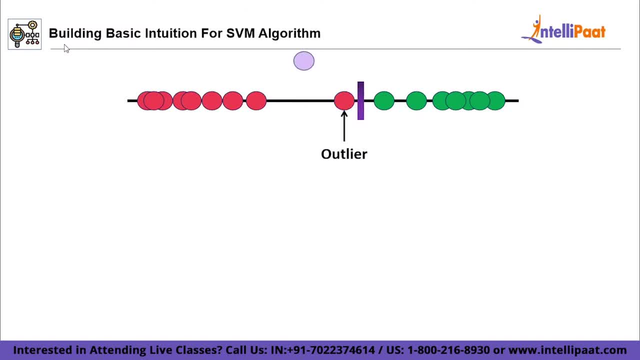 In this case, maximum margin classifier will be too close to the obese cluster and really far from the observations that are not obese. Now, if we get new observations somewhere around here- the purple dot that I am referring to- we would classify it as non-obese even. 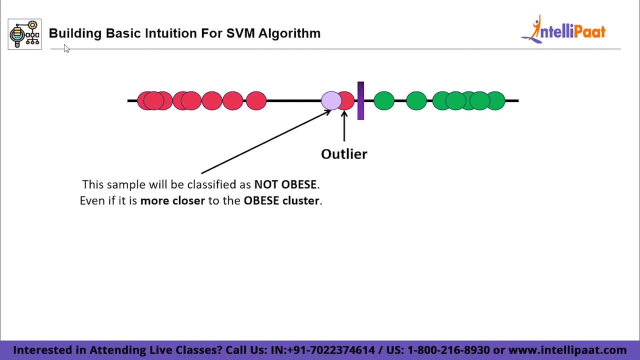 though most of the non-obese observations are much further away than the obese observation. So from this we can deduce that these maximum margin classifiers are super-duper sensitive to the outliers in training data, and that makes them pretty lame. I hope you guys have. 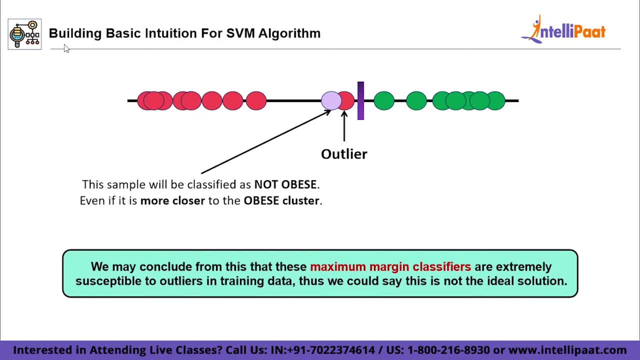 got what I wanted to convey to all of you. Now this is again a problem, and can we do anything to overcome this? Can we do more better? Well, yes, to make a threshold that is not so sensitive to outliers, we must allow the misclassifications. For example, if we 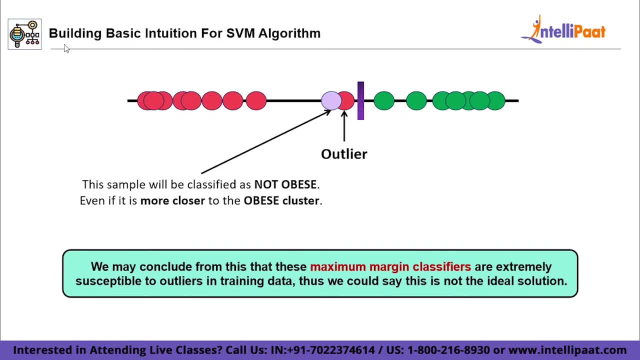 put the threshold halfway between these two points, we'll for sure misclassify this particular observation. However, now when we get a new observation here, we'll classify it as obese, and this makes sense because it is very closer to the most of obese observations. 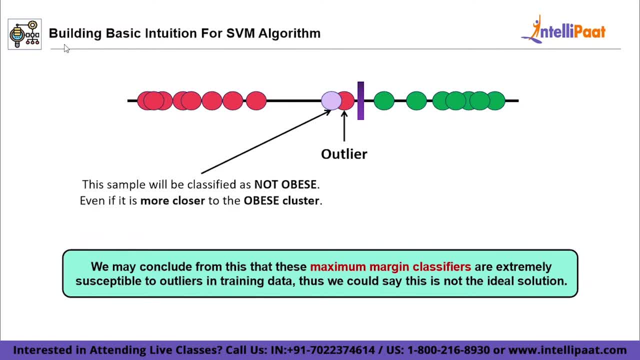 Choosing a threshold that allows misclassification is an example of the bias variance trade-off that plagues all of the machine learning. In other words, before allowing the misclassification, that is in case of maximum margin classifiers, we picked the threshold. that was very sensitive. 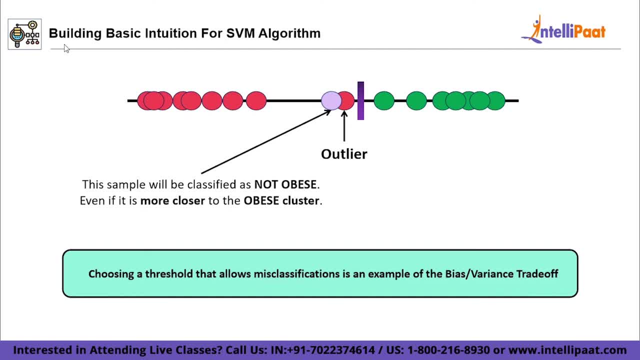 to the training data. It had low bias And it performed poorly when we got new data. In contrast, when we picked the threshold that was less sensitive to the training data and allowed misclassification, so it would have a higher bias and it would perform better when we get new data And somewhere that is. 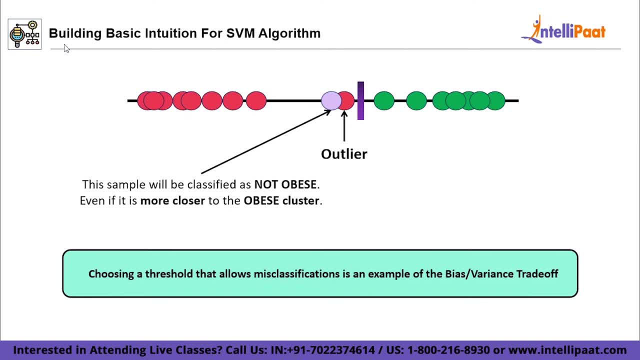 the reason why it will have very low variance. Now, this was some technical jargon-ish stuff that I just discussed. Basically, guys, when we allow misclassification, we should allow the misclassification. that is, in case of misclassification, the distance between the observations and threshold is called. 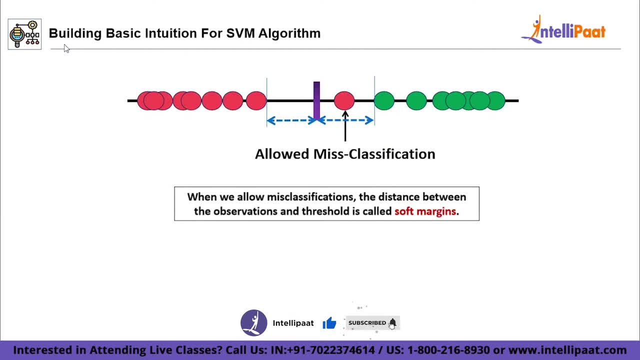 as soft margin. now the question that stands here is that: is this soft margin a better technique? the answer to this question is pretty simple. we use cross-validation to determine how many miscalculations and observations to allow inside of the soft margin to get the best classification. for example, if 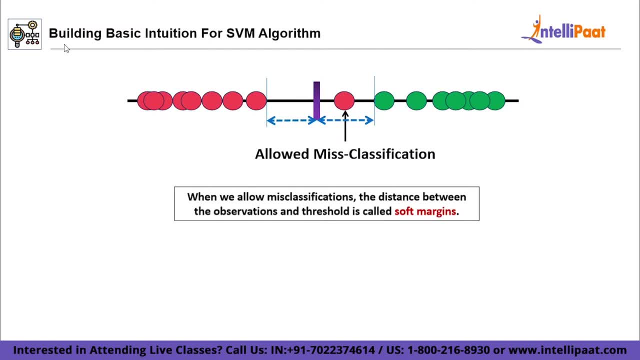 cross-validation determined that this was the best soft margin, then we would allow one misclassification and two observations that are correctly classified to be within the soft margin. when we use a soft margin to determine the location of threshold, then we are using the soft margin classifier, or what? 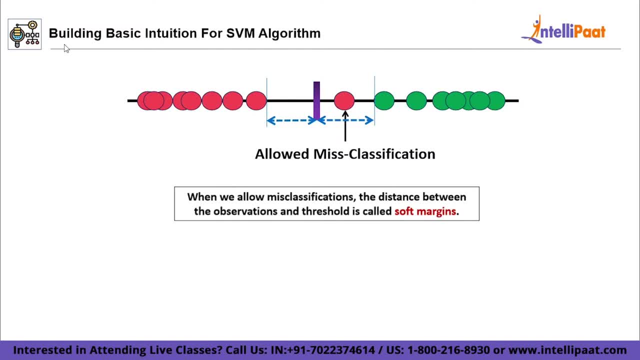 we call support vector machine. in general machine learning terms, the name support vector machine comes from the observations at edge and within the soft margin. these observations are classified as soft margin and the situations are called support vectors in machine learning terminology. hence the name support vector machine. now let's say we have two features given that are: 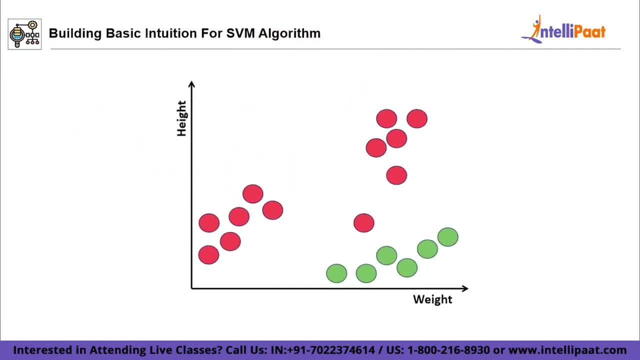 height and weight. and now, if we plot them, the graphical representation will be two-dimensional. right and now, if I were to formalize the support vector machine classifier for this particular sample, I'll focus on these two points. right. these two points will be called that support vectors and based upon them, I'll find 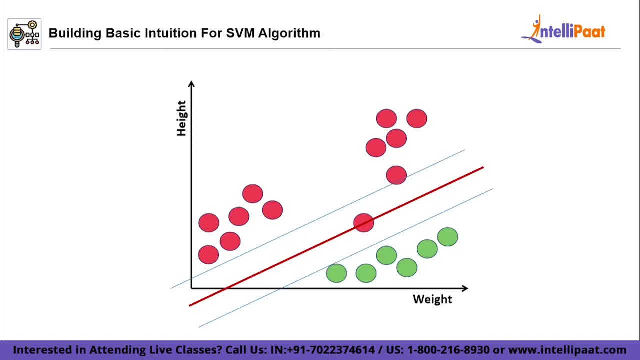 this average classifier. alright, these two light blue lines are nothing but the lines that are giving us the sense of where all of the other data points are with respect to the soft margin classifier that we just have found out. in machine learning terms, these lines are called as hyperplanes. basically the main. 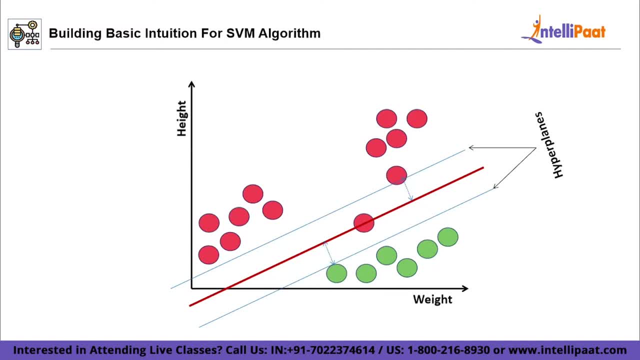 classifier will sit in the middle of the data points and we are going to see both these hyperplanes. Now let's say I have a three-dimensional data In this particular sample. let's say I do have BMI feature as well. Then our graph will become three-dimensional. 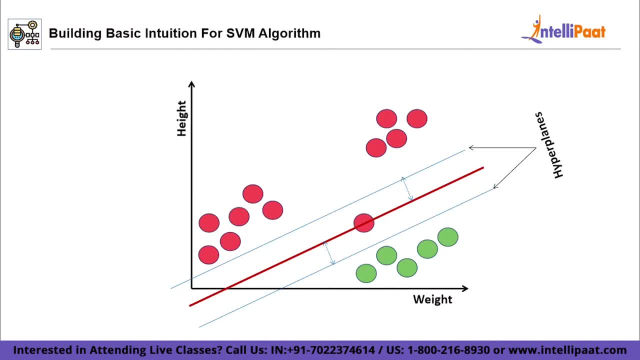 alright, and the classifier will not be a line. instead it will be a three-dimensional plane. So technically, if I have to boil down the algorithmic formulation of a support vector machine, I would say we use the SVM technique to discover the points from both classes that. 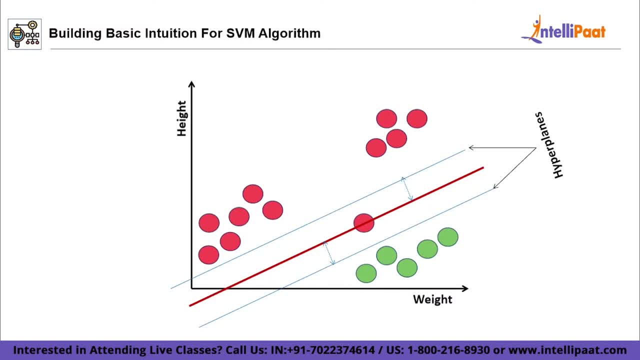 are closest to the line. These points are known as support vectors. Now we compute the distance between the line and the support vectors. This distance is called as the margin. Our goal is to maximize this margin, and the hyperplane for which the margin is maximum is the optimal hyperplane. 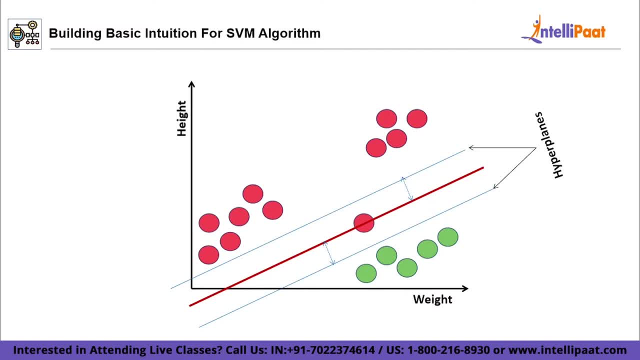 And this SVM tracks many adventure planes in its transformation tries to make a decision boundary in such a way that the separation between the two classes is as wide as possible. But not only that. these support vector machines make use of kernels to convert given data into a three-dimensional plot so that it could find a plane that can. 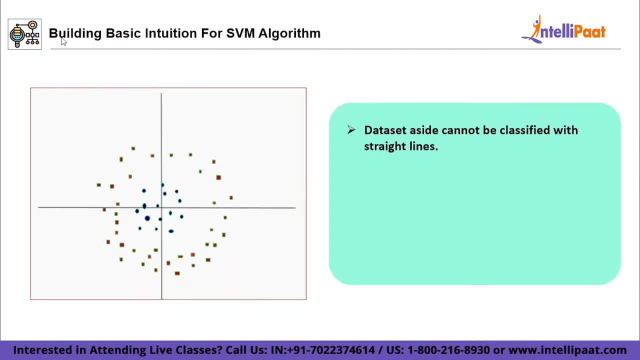 classify the data points. Check this example given right here. These data points cannot be separated with the help of straight lines. We'll need a circular classifier to do that, and the equation for same will be in the format: z is equal to x square plus y square, and. 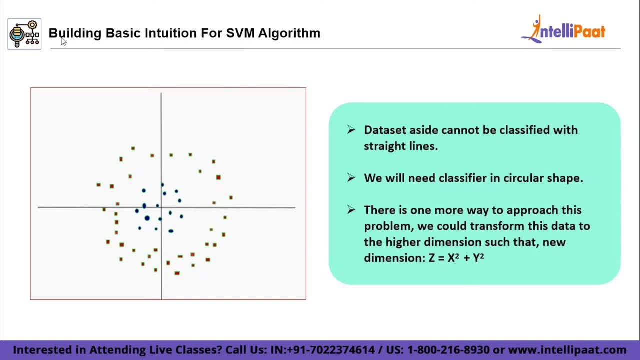 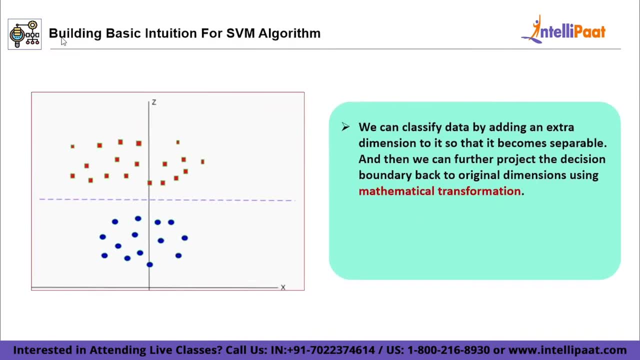 I can simply achieve that by just including one more dimension. The same data will look something like this on z-axis, and it can be easily classified with the help of hyperplane. From this concept you can make a note that we can classify data by. 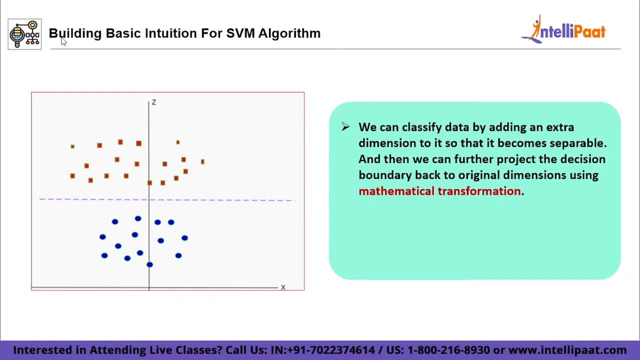 z-axis, and it can be easily classified with the help of hyperplane. From this concept you can make a note that we can classify data by adding an extra dimension to it so that it becomes linearly separable, and then we can further project the decision boundary back to original dimension using mathematical. 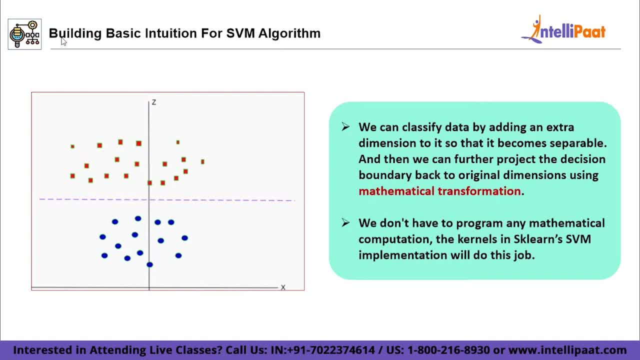 transformations, But finding the correct transformation for any given dataset is not that easy. Thankfully we can use kernels in SKlearn's SVM implementation to do this job Basically. you don't have to scratch your head for the mathematics that works behind the support vector machine. 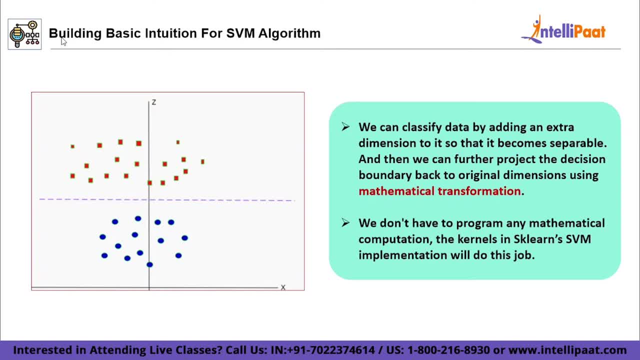 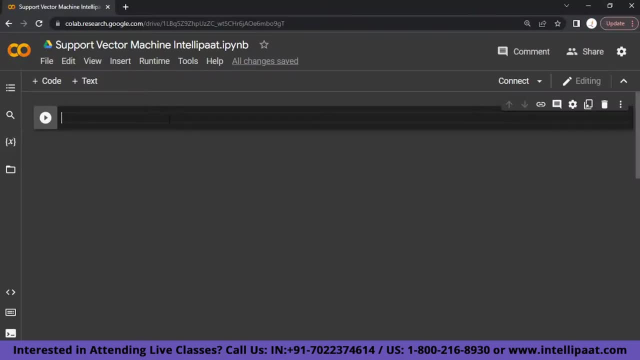 Alright, I hope this theoretical concept of a support vector machine is clear to all of you guys. Now, moving ahead, we'll visit the code editor and develop one support vector classifier with the help of scikit-learn library. Alright, guys, the dataset that we are going to use for understanding the function of SVM. 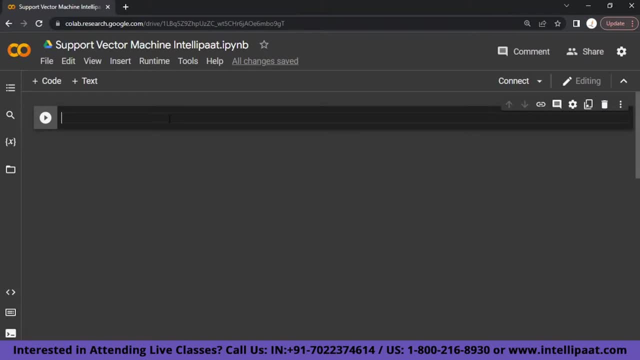 is the iris dataset that we have discussed in previous sessions as well. So to get this data loaded into our directory, let's first import few dependabilities, right? So first I'll import numpy as at: N6040ined, directed at 0 to d1, contained library. 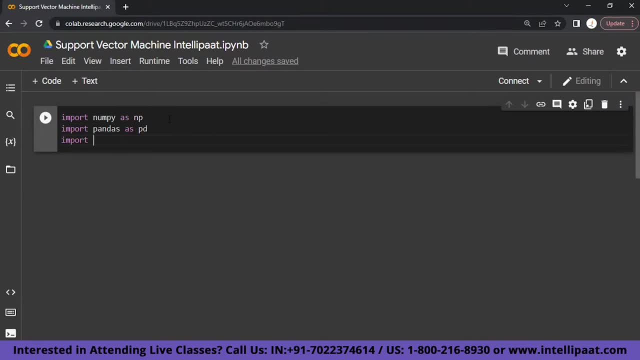 Next we'll import matplotlib script floating property. Then we'll import the dataset's framework from SKlearn הכ, meaning from SQL. on import data sets: all right now, let's run this block. now in the next step, what we'll do is we'll load our data from the data sets framework of. 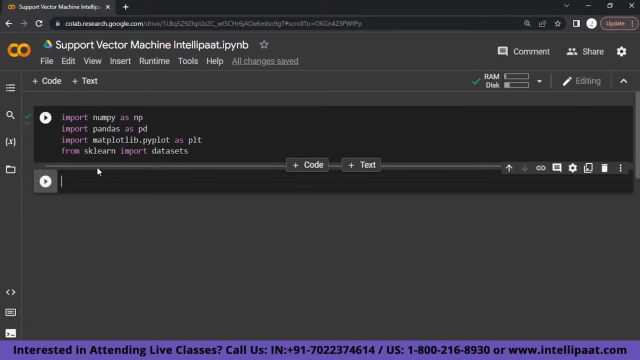 SQL on. the function that we are going to use is load underscore iris, so let me load this data quickly. iris will be equal to data sets. dot. load underscore iris. now let me run this block as well. now, next thing we will do is will separate features and targets into X and Y. X will store the features, whereas Y 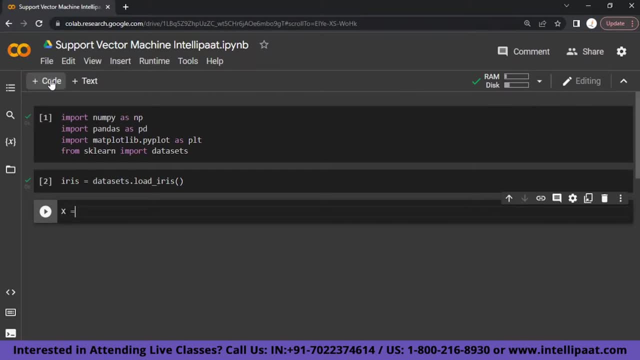 will store the target parameter, so we'll put X is equal to iris dot data and we will add y as iris dot target and also we will set names that are the names of entries as iris dot target underscore names, and I will run this block. Now, if I want to show you guys x dot shape, I could do that with this command and similarly. 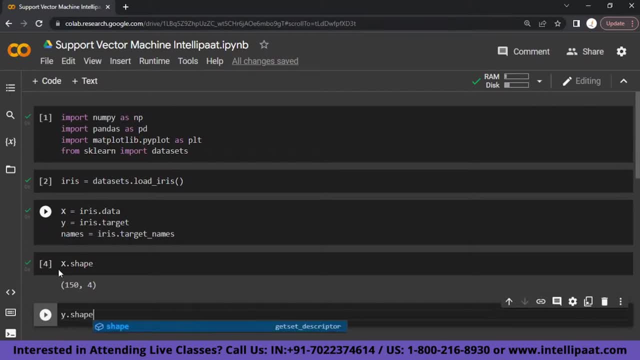 for y dot shape. Now, guys, I could have used returns, Return underscore x, underscore y- parameter to get the data into x and y variables. But instead of doing that, we want to create data frame where we will have both data and label together so that, with the help of plotting, we can visualize how our data can be classified. 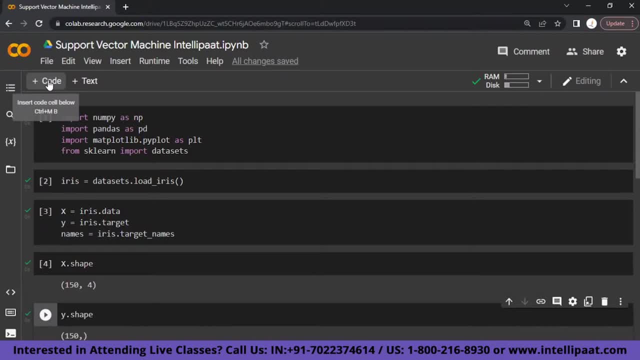 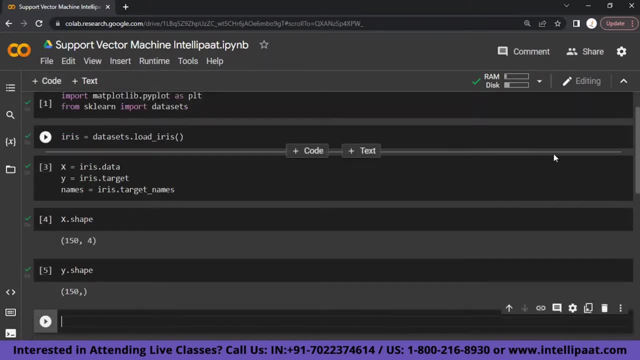 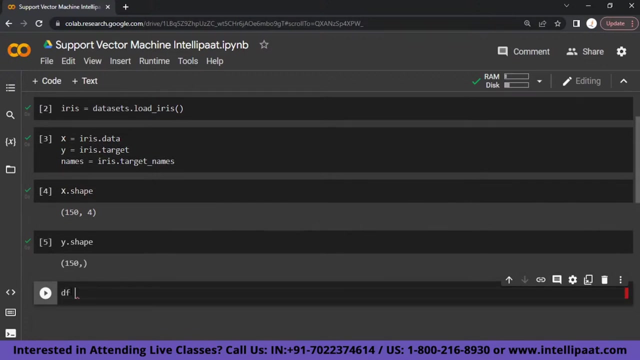 Now let me create that data frame and inside it I'll store the features and will also set the column titles to feature names. Now, to do that, let me get the new block here Now. First of all, we'll create the data frame. df is equal to pd, dot data frame inside it. 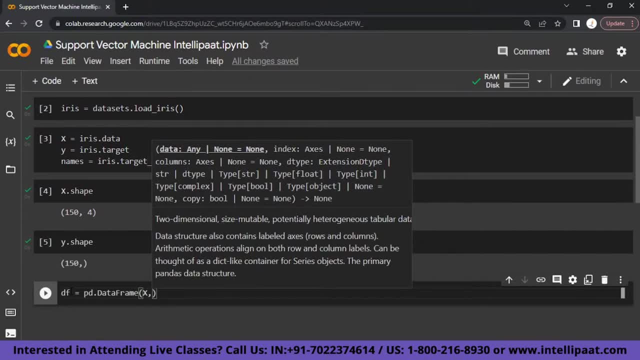 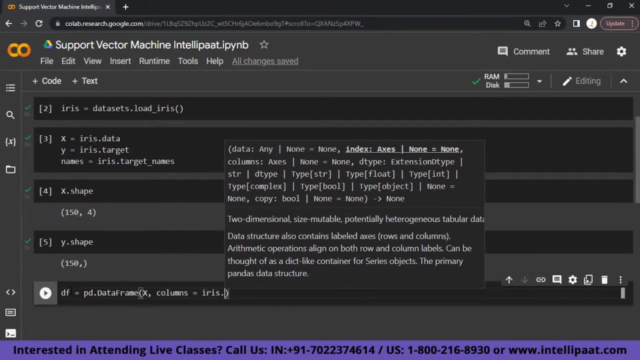 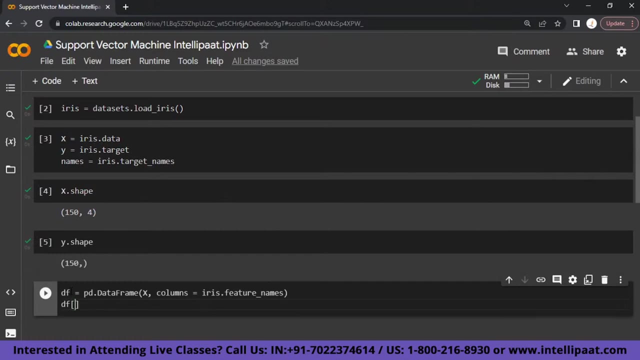 I'll pass the input, that is feature, and I'll set columns as iris dot feature names. next, I'll set The target variable as species and I'll add it to our data frame and the entry will be nothing but the target. Next, I don't want our targets in numerical format because I want to visualize data and 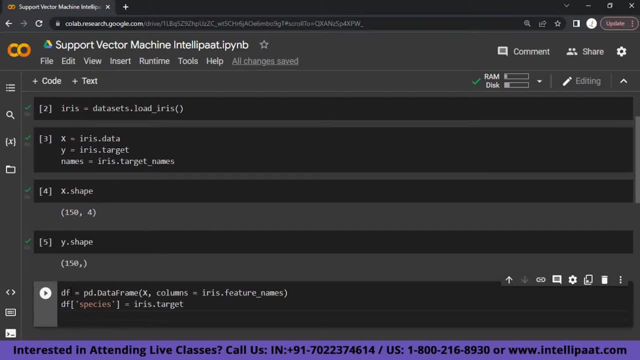 I want to know which class the objects belongs to and how they look. all right. So, for that purpose, what I'm going to do is I'm going to set flower species title As setosa, versicolor and virginica, which are the three classes that we have in iris data. 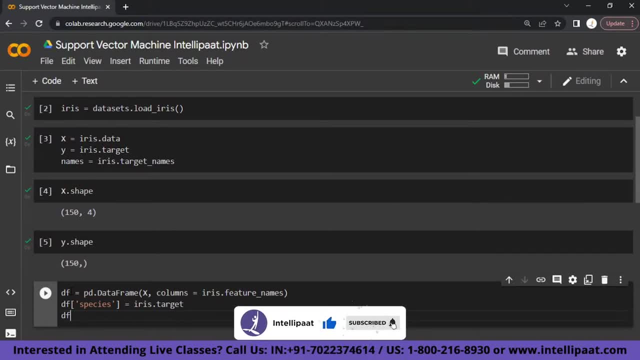 set. All right, and to do that I'll write command df species will be equal to df species. dot replace and will replace them to zero comma one, comma two To value. So Setosa, versicolor and virginica. Now let me run this block. 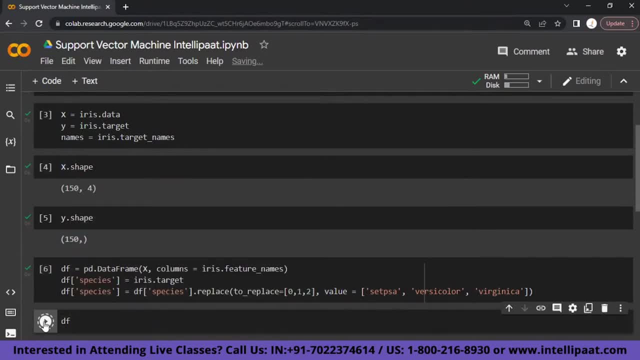 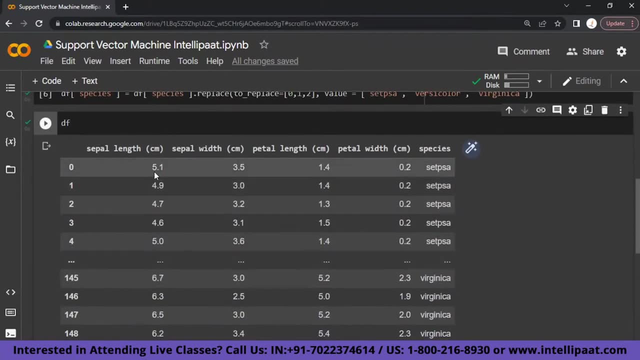 Next, I'll print the data frame so that we'll be able to visualize how our data frame actually looks like. all right Now. here you can see that we have sepal length, sepal width, petal length, petal width, And we can see that. 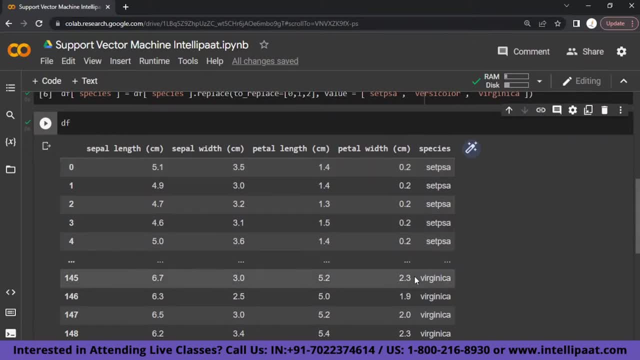 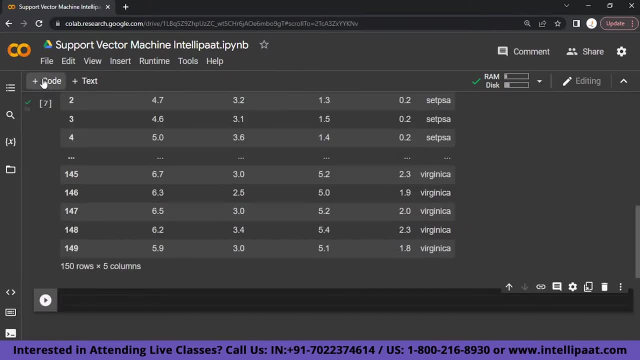 And species In Naming format, not in numerical 0, 1, 2 class format. all right, So now that we have our data together, The next thing we want to perform is eda, That is, exploratory data analysis, And let me tell you, guys, that we have one of the most powerful method available in seaborn. 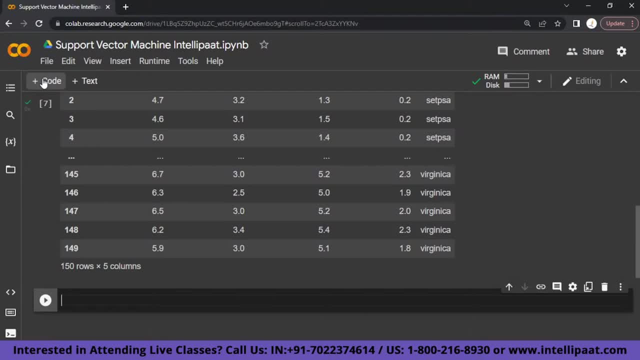 that can allow us to do the rapid eda. Now, in order to use this functionality, Let me first import the seaborn library, all right. And then, in order to do this functionality, to import the data library to the seaborn library, right? so import seaborn as SNS. now the functionality that I was talking about. 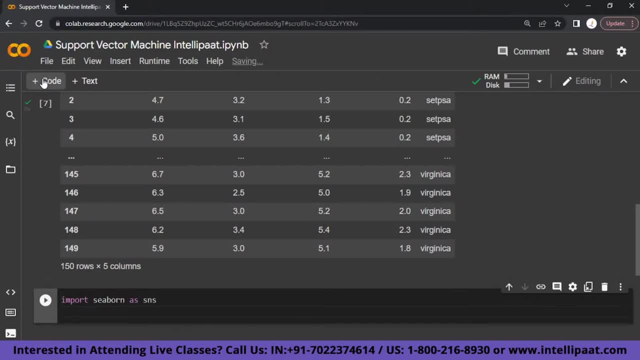 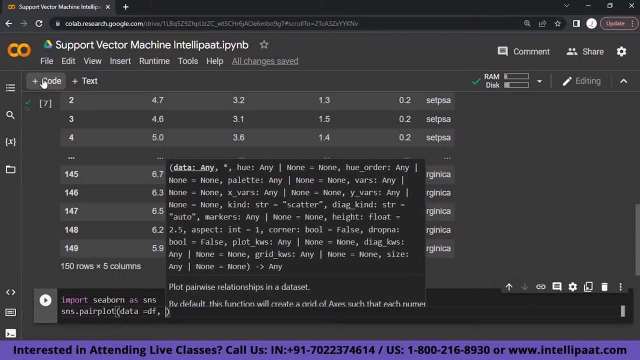 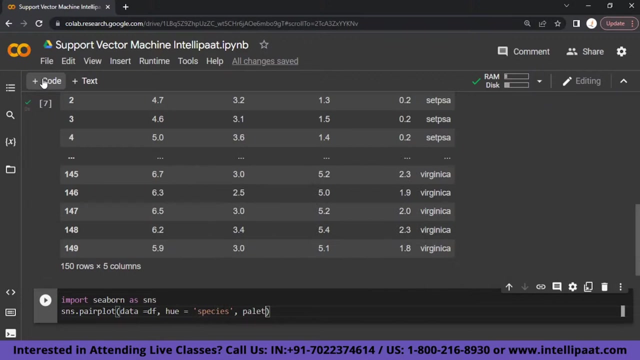 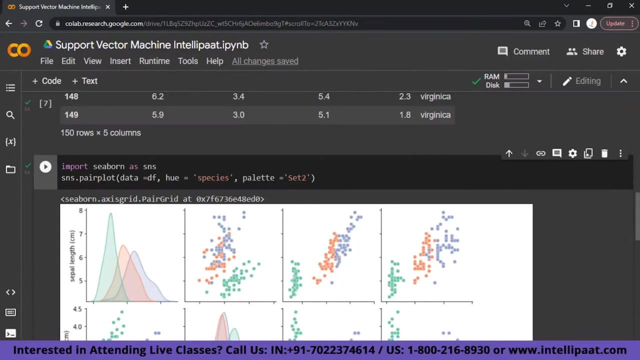 is nothing but the pair plot. so let me also create this pair plot, so SNS dot pair plot and I'll pass data as DF, I'll set you adds species and we'll set Palette ads. set to now. let me run this block now. here you can see multiple. 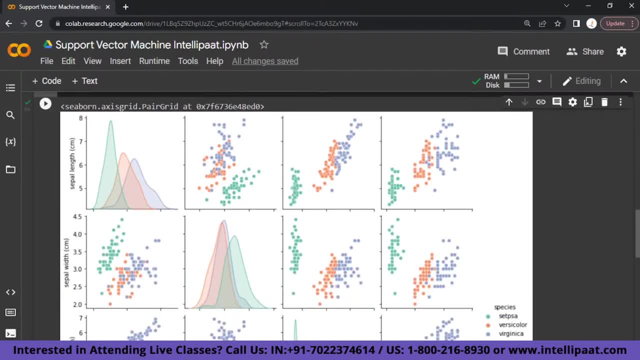 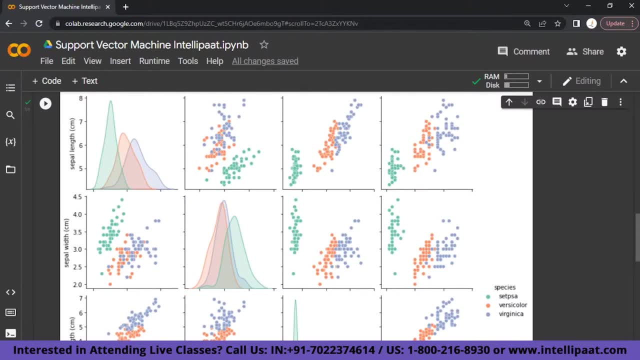 plots that are actually showing how our data is distributed. alright, so this is our data distribution. we also have our fields here that we need to. So, basically, guys, this pair plot function includes two main graphs, such as scatter plot and density graph. The density graph on the diagonal allows us to see the distribution of a single variable. 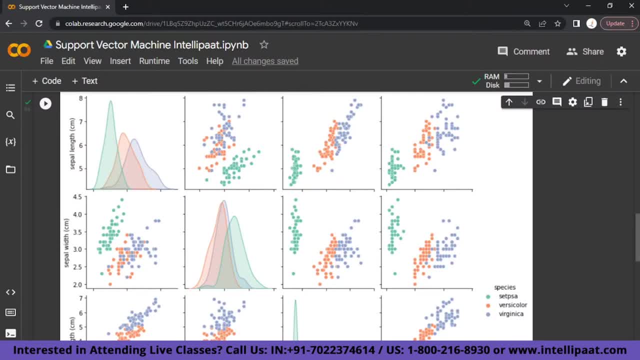 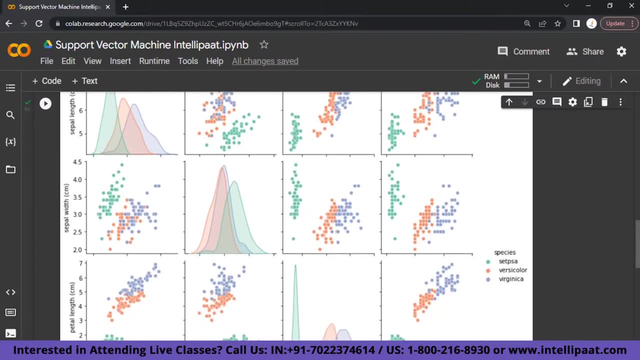 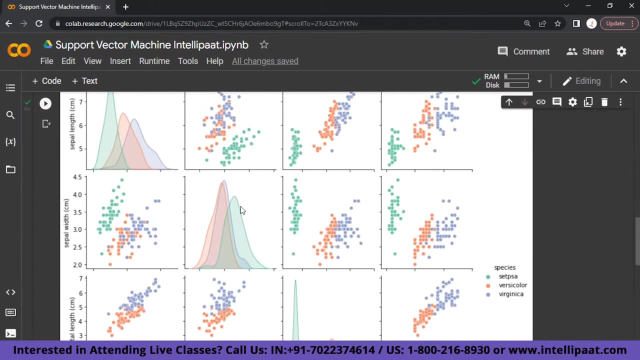 while the scatter plots on the upper and lower triangles show the relationship between two variables. all right, Now, here you can see that we have these distribution graphs on diagonals, all right. So, basically, these are the graphs that are showing how our data is distributed. and then 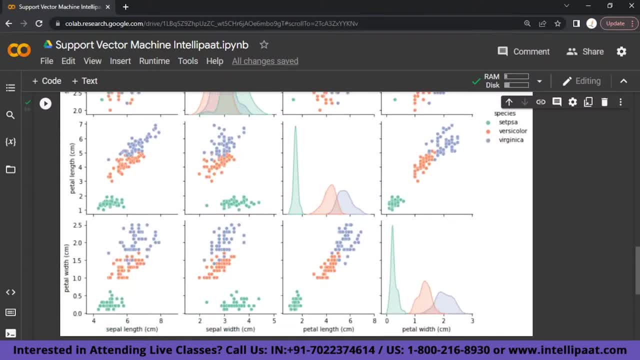 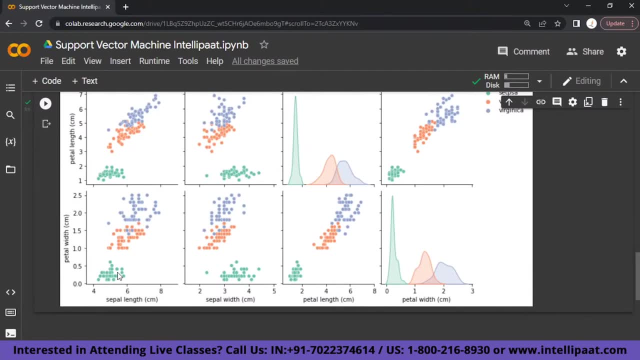 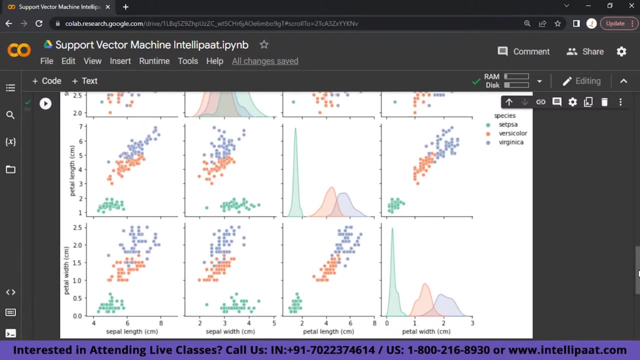 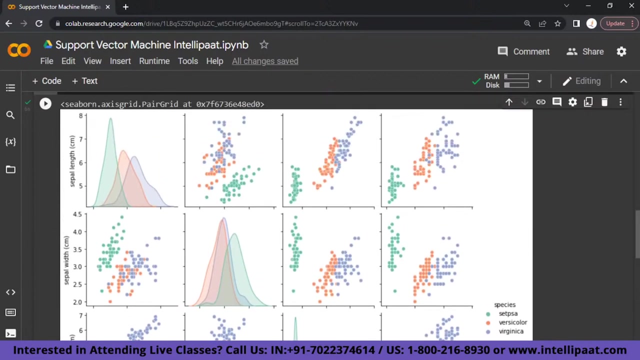 we have scatter plots Now. this scatter plot at downside is against petal width and sepal length, and we have green as setosa, then we have red as versicolor and purple as virginica. all right, Now from here you can visualize that how we can classify our data with multiple lengths. 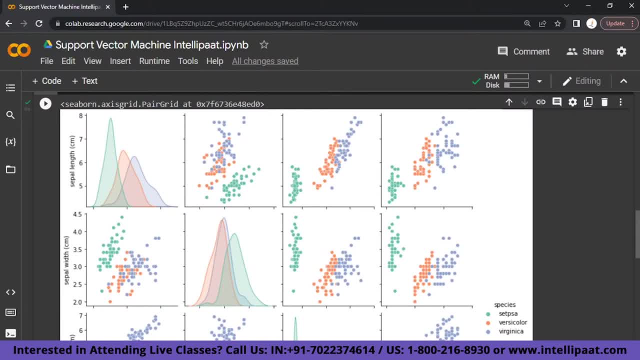 Single lines, or, in fact, we cannot classify this data with a single line. for that purpose, we are gonna required some sort of hyper plane, or we need to transform this data into three dimensions. all right, and for that purpose we have support vector machine algorithm. Now, before we apply support vector machine, first of all we'll need to split this data. 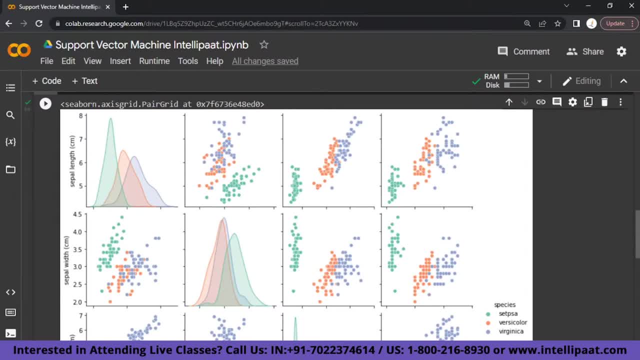 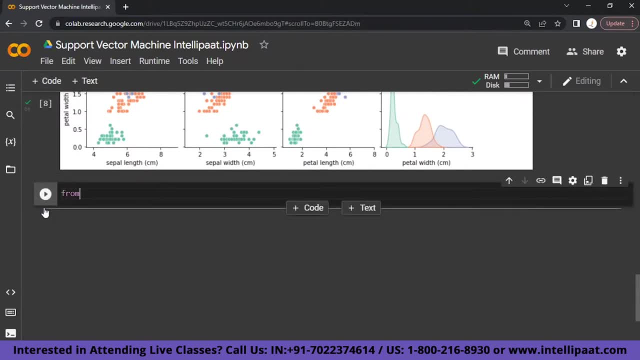 into training and testing samples and for that purpose I'm gonna import the train test split functionality. Now the syntax to do that is from sklearn dot model underscore selection, import, train underscore, test, underscore split. and next thing I'll do is I'll transform our data into: 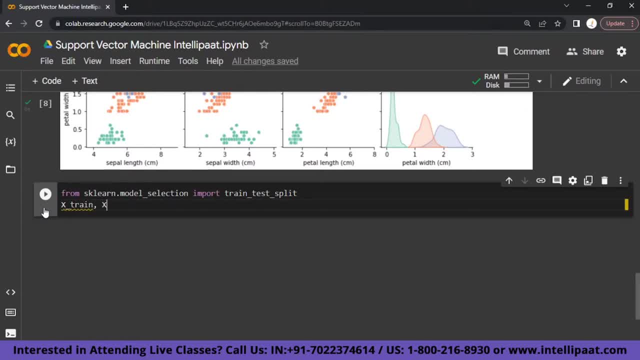 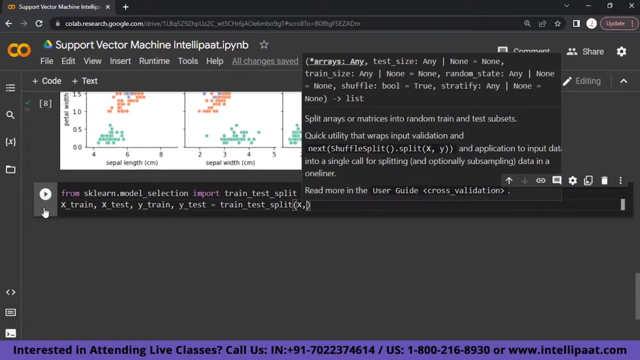 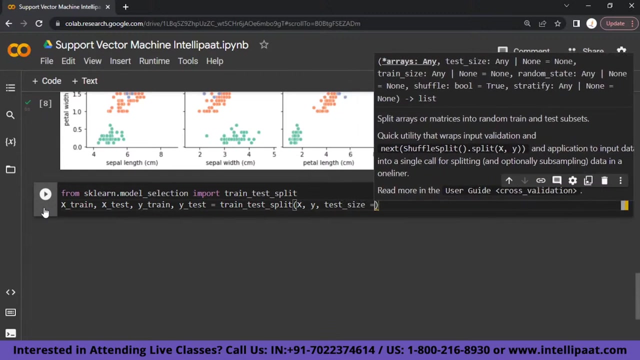 training and testing sets. So x, train, comma x underscore test, comma y, train, comma y underscore test is equal to train underscore test, underscore split, and I'll pass, and I'll pass feature vector, the label vector, Then the test size. Now, guys, we do have very less samples in this iris data set. 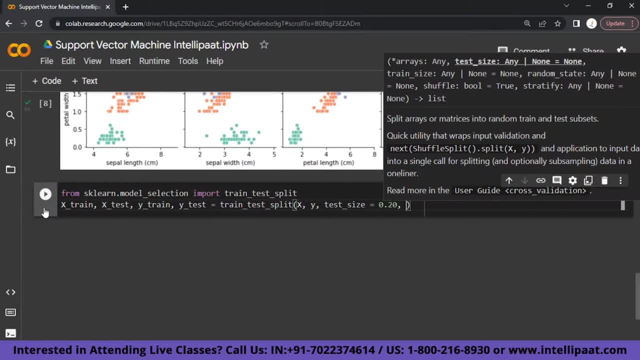 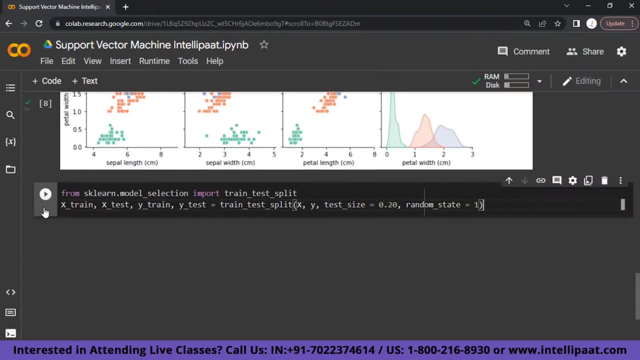 So we'll set test size as 20 percent and we'll set random state as one. Now let me run this block. all right, Now we do have training and testing samples differentiated, all right. So let me print the sizes for training and testing. 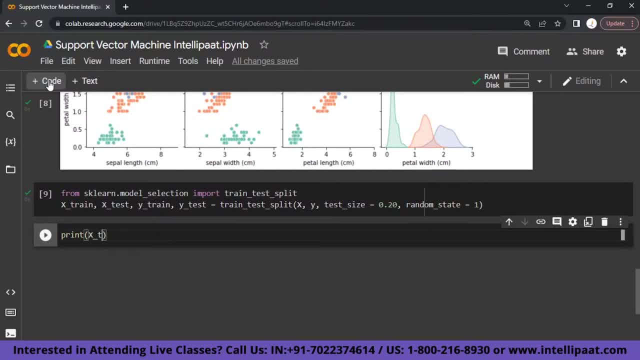 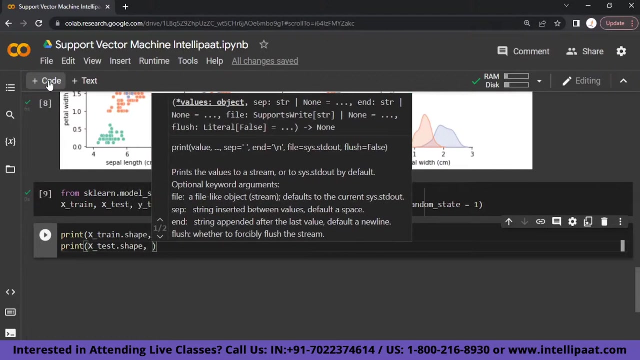 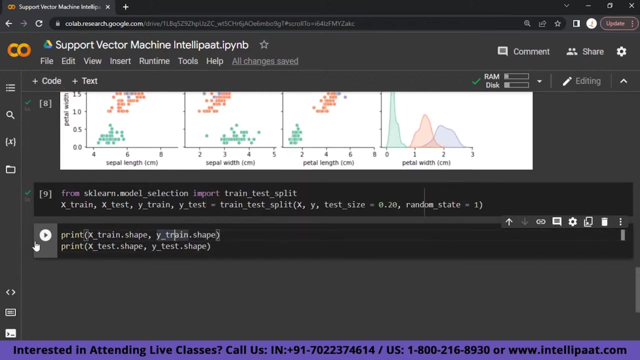 samples one by one. So print x underscore train dot shape, comma y underscore train dot shape and similarly I'll print the testing data set sizes, that is, x underscore test dot shape, comma y underscore test dot shape. Okay, Let me run this block, all right. 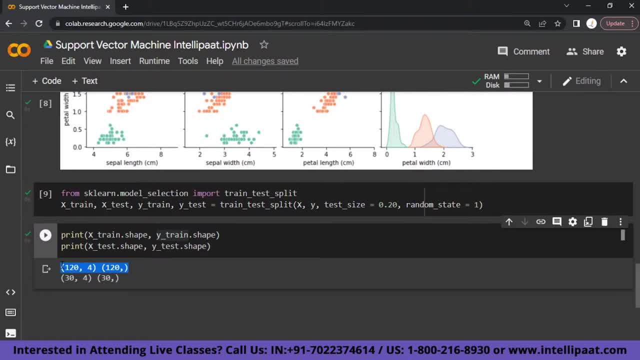 Here you can see that we have 120 samples in our training data set and 30 samples in our testing data set. all right, Now the next step will be applying the support vector machine. first of all, I'll need to import the support vector machine algorithm from sklearn, and the syntax to do that is from: 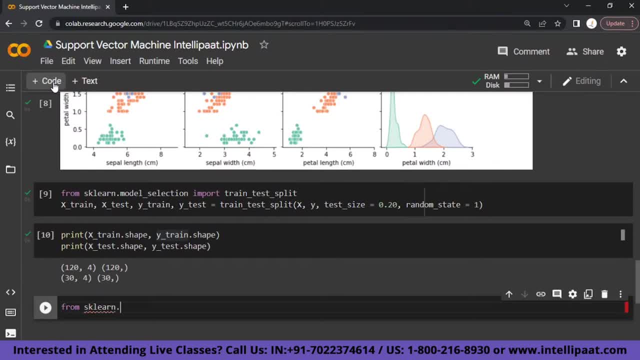 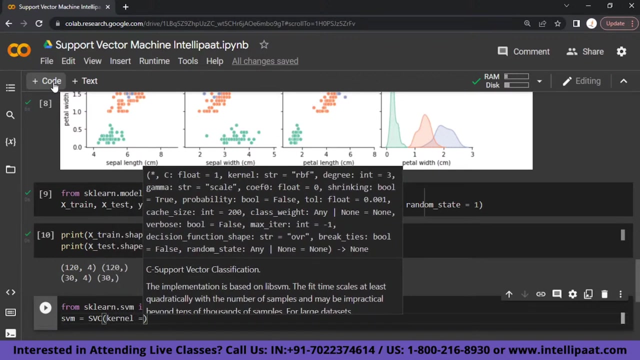 sklearn. Okay, So I'll take my stdsvm import svc Now I'll set svm as new object and I'll add the functionalities of this svc to it. Now the kernel that we are going to set for first observation will be linear and the random 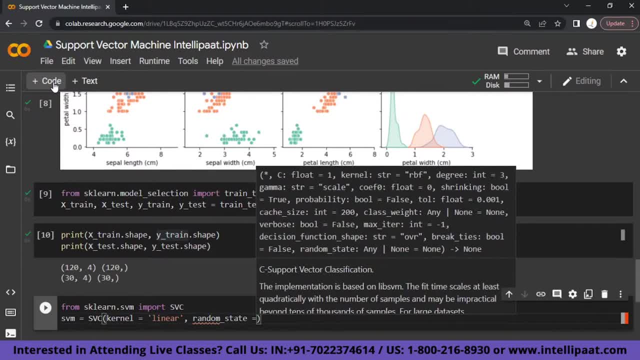 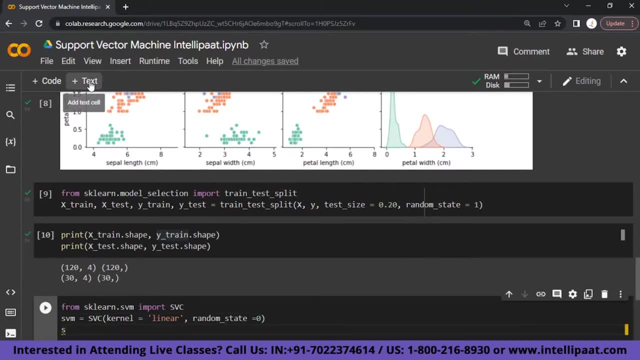 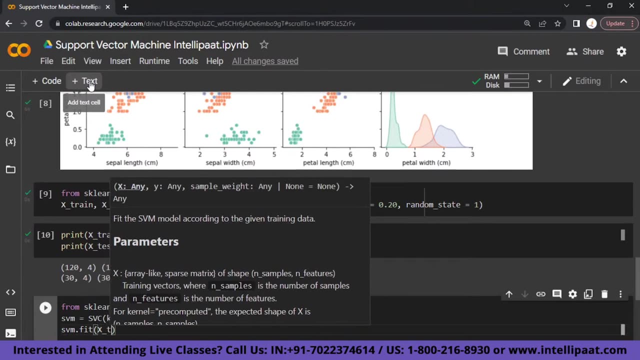 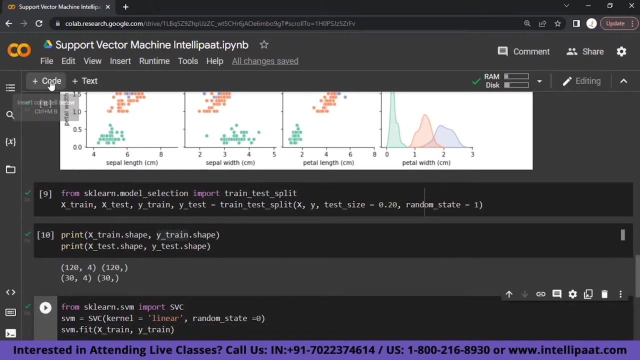 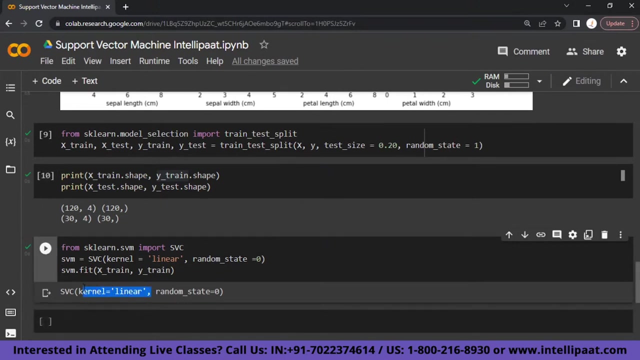 state Okay will be 0.. Now we'll fit our data to this model, that is, svm object. dot fit x underscore train. comma y underscore train. Now let me run this block. Now we have successfully created the svm object with linear kernel. All right, guys. Now we want. 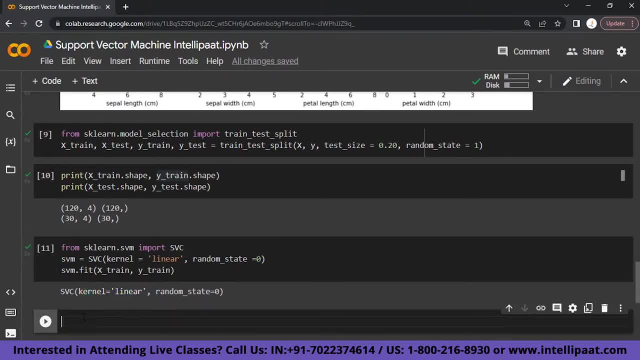 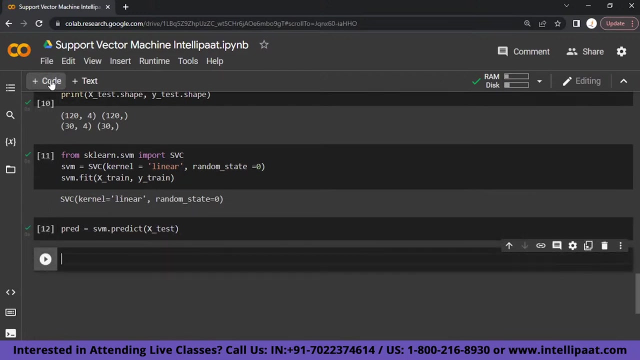 to see how our model is making predictions. So let us make predictions and store them under the thread vector. So svm dot predict x underscore test will be stored inside thread. now, once I run this block, those predictions will be stored inside this thread variable. now, if I want to visualize them, I can. 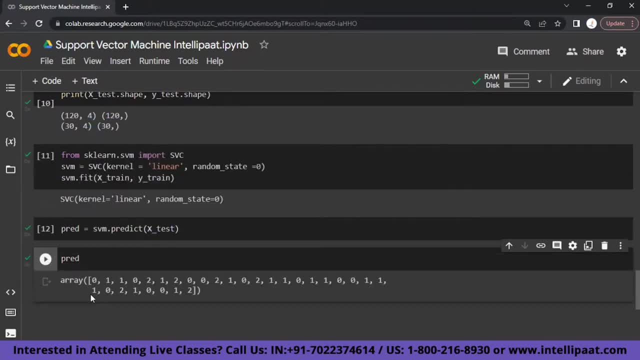 simply type thread here and our results will be printed over here. now next thing I want to visualize is the accuracy of our model. so for that purpose, what I'll do is I'll import the accuracy score metric from sklearnmetrics framework. for that purpose, I'll write command from sklearnmetrics. 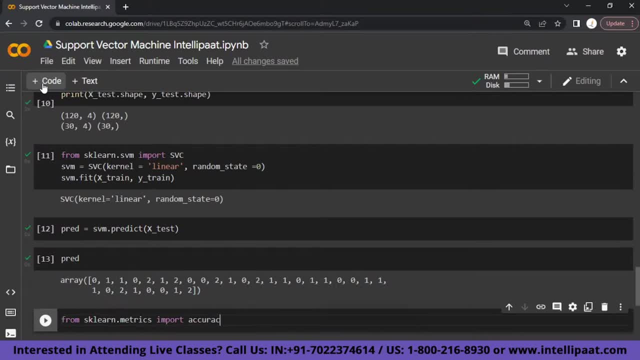 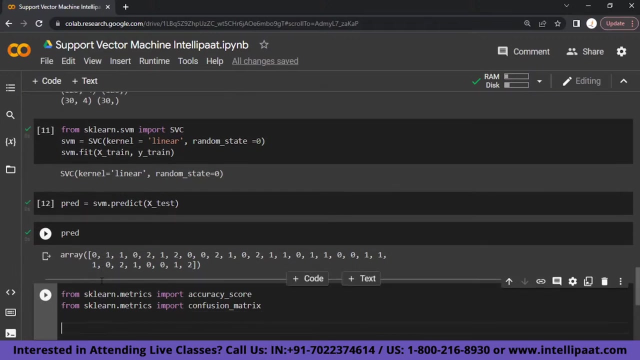 import accuracy underscore score and similarly I'll also import the confusion matrix to visualize the accuracy and the misclassifications made by our model. so confusion underscore matrix. now the next thing I'll do is I'll apply this accuracy underscore score functionality to our testing sample and made 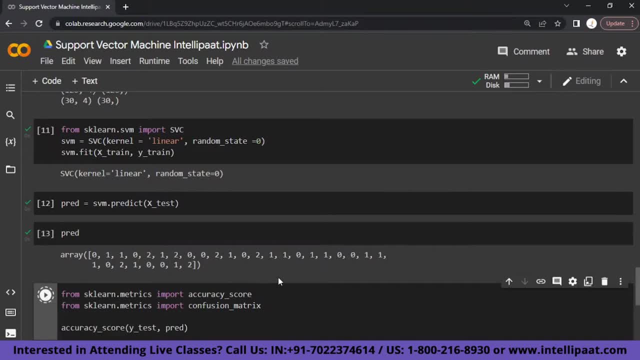 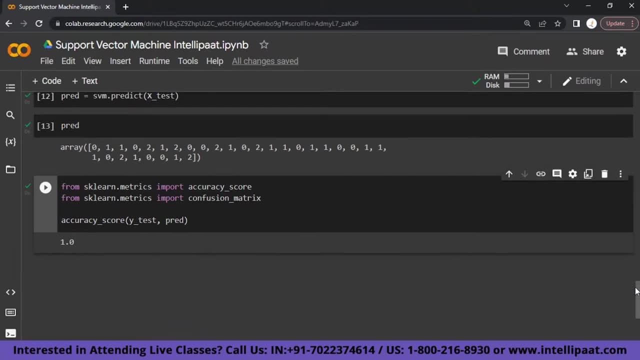 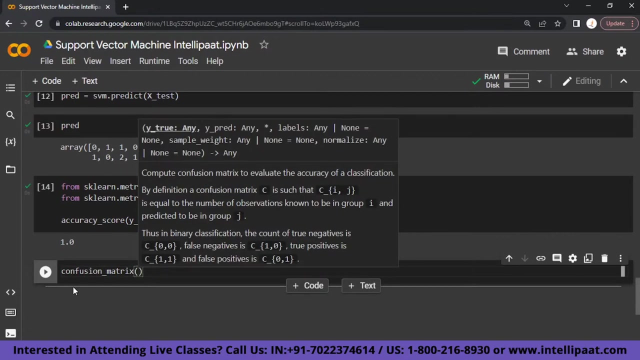 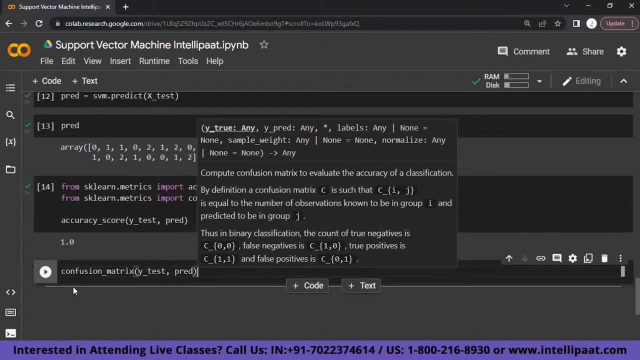 predictions. alright, guys, and this will return the accuracy of our model, and that is one that means our model is not missing, misclassifying any data sample. alright, similarly, if I want to print the confusion matrix, I could use the function confusion underscore matrix. I could pass parameter y underscore test comma predictions. and here, since there, 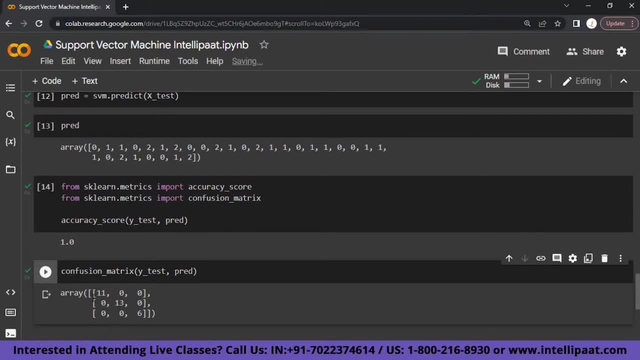 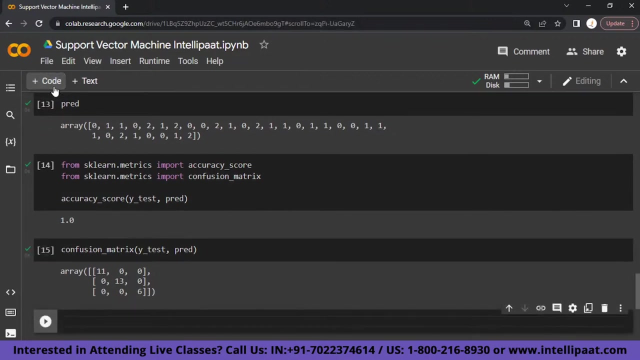 is no true positive or true negative values available over here. our model is set to have precision of 1, that is 100% accuracy. alright, now let's say we want to use another kernel for this purpose, so let me create the another kernel, the kernel that we are going. 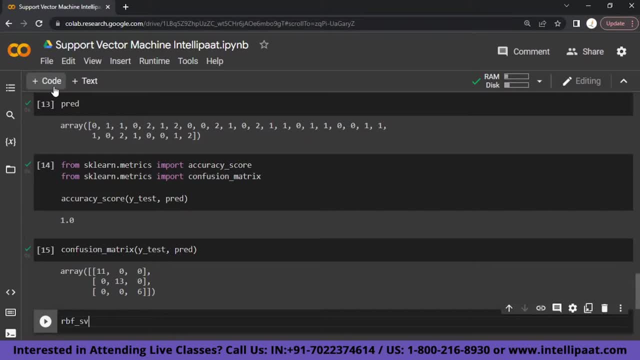 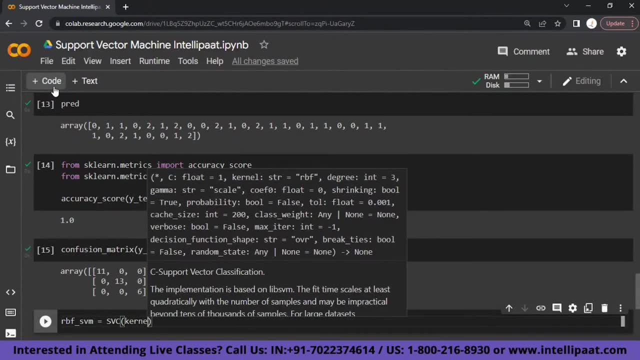 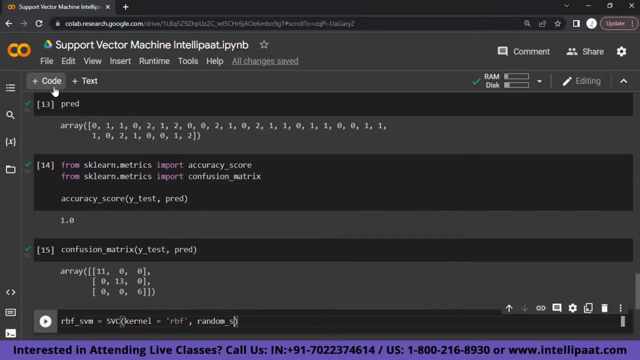 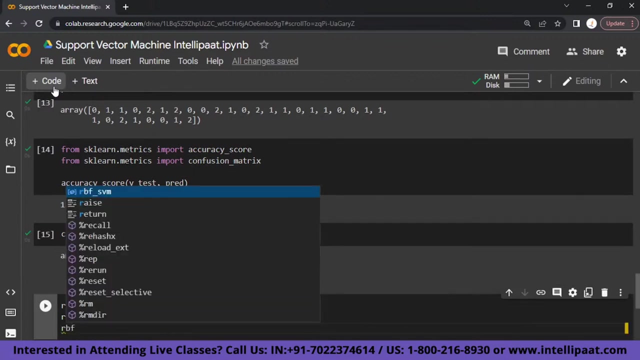 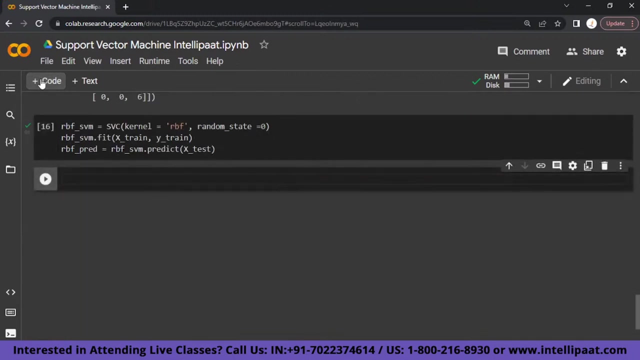 to use is R B f, so R B f underscore SVM. we will store the SV c object where kernel will be set to our revolt End submit, End submit And again we'll keep random state at zero. We'll fit our data to this RBF kernel SVM model and we'll make prediction as well. 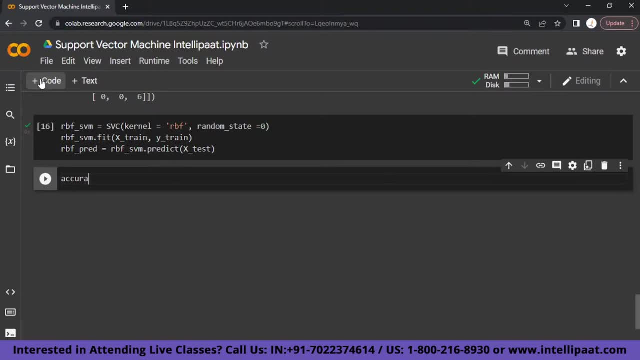 Now let us print the accuracy for this particular kernel. Okay, And here you can find out that we are getting accuracy of 96%, alright, which is again a better accuracy, but since radial basis function is transforming our data into multiple dimensions, and with linear kernel we are actually getting accurate results, and with RBF we are not getting- 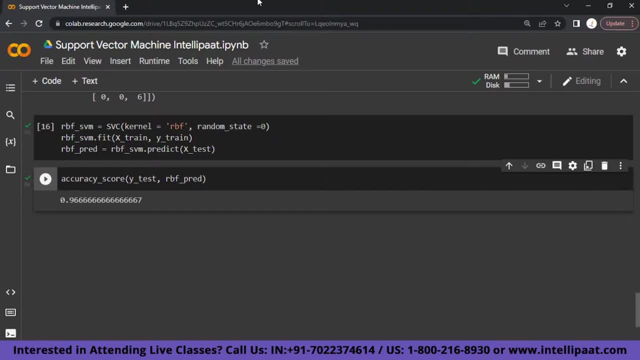 the accurate result in this case. This time that is 100% accuracy. but 96% accuracy is again a very good accuracy, guys. And in some cases linear kernel won't suffice for the data, but in those cases RBF can do wonders and sigmoid can do wonders. 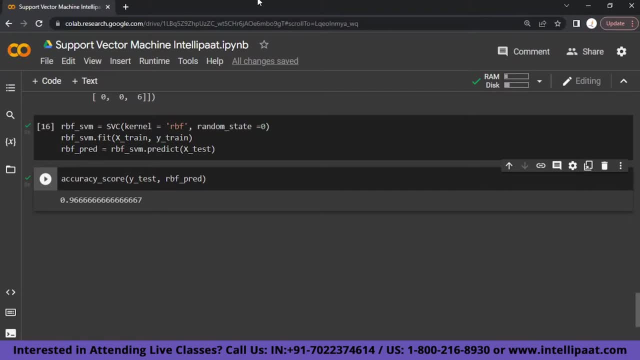 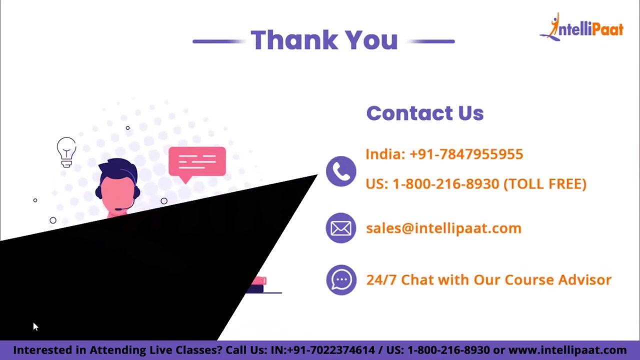 So, similarly, you can try multiple combinations of SVM kernels and try how these different kernels are working and how these different kernels are producing outputs on different datasets. Alright, Okay, guys. I hope the concept of support vector machine is clear to all of you guys out there.